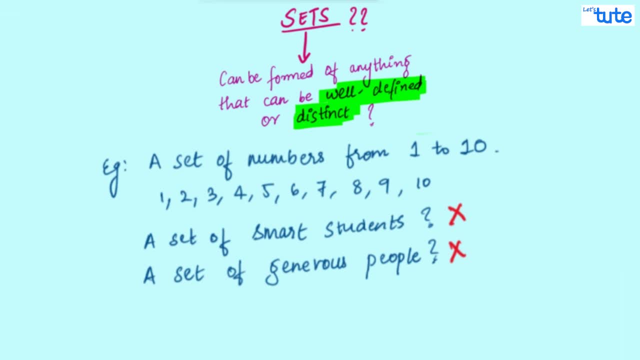 smart students. Can this be considered as a set? No, not exactly right, Because here smart or generous cannot be defined or measured. or we can say that these are relative terms, because the meaning of these words will change from individual to individual. Hence we cannot. 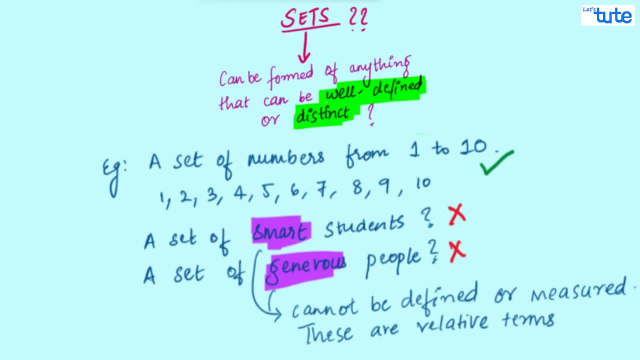 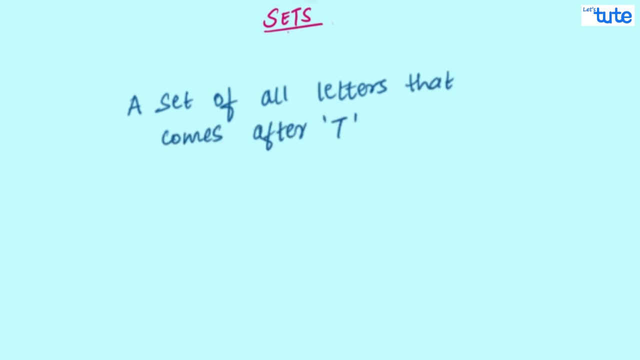 make a set of these situations. Let's take a simpler example: A set of all the letters that comes after T. So what all letters will be there? U, V, W, X, Y and Z? Yes, so this can be also called as a set Right. Let's see few of these examples. if we can form a. 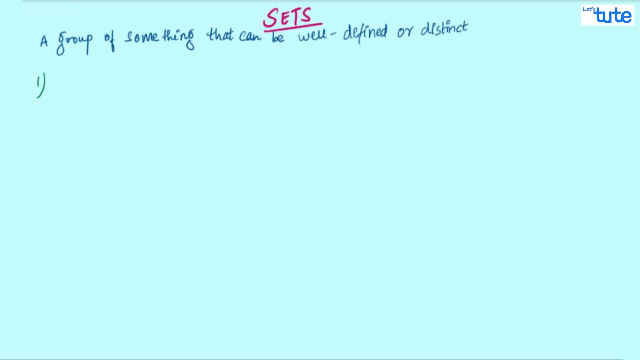 set of them or not? The first is states of India. So can we form a set of this? Yes, because there are 29 states of India, So there are 28 states of India. Okay, So let's 29 states in India, and you can list all of them. 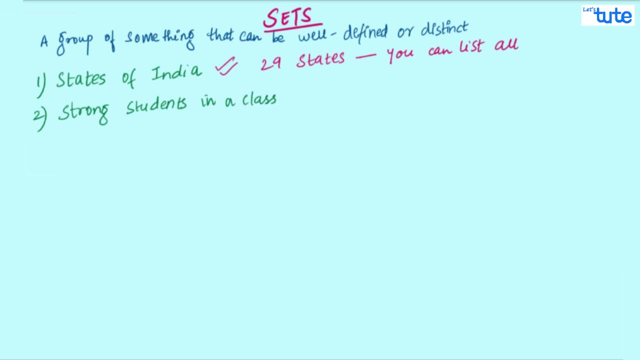 The second one is Strong students in a class. Well, this cannot be a set, because strong is a relative term, But suppose here, if I'll add a condition, like students who weigh more than 50 kg in a class are to be considered as strong. 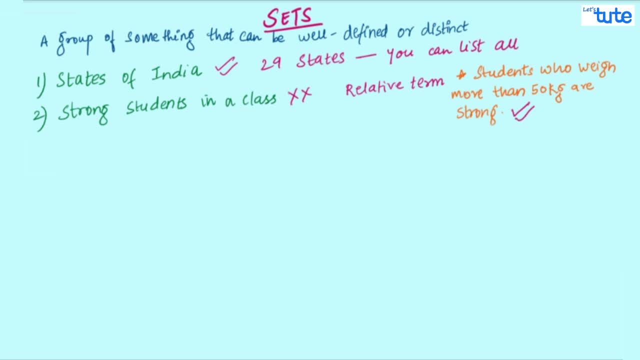 Can now this be formed a set? Yes, because now we have a number, a quantity or a well-defined and distinct property that we can use and form this set Right. Let's see the next one: Students who have scored 70% and above in the last semester. 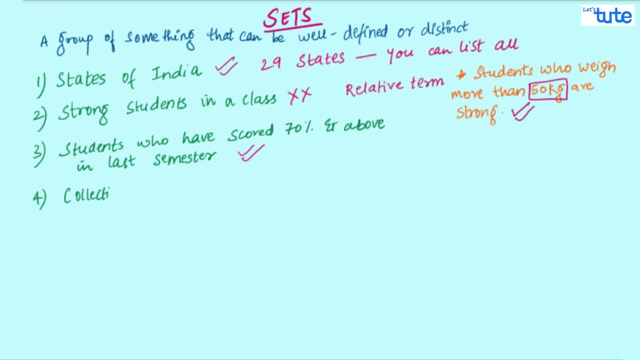 Yes, you can form a set of this Collection of great people in the world. Again, great is a relative term and we cannot form a set of this. So I hope by now you know what are sets and in which conditions we can form a set. 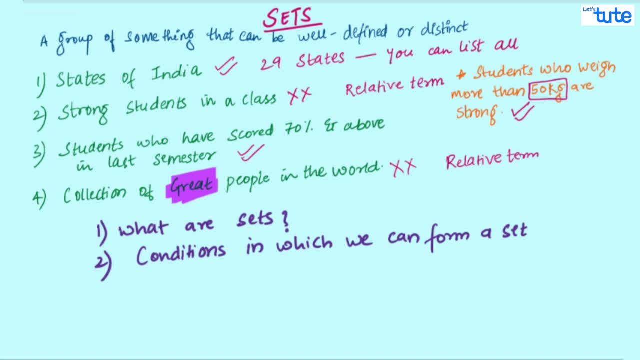 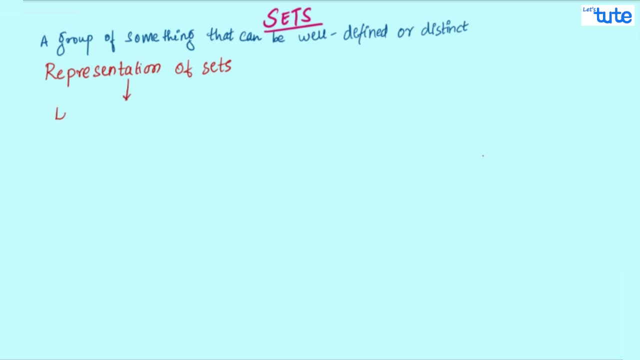 and cannot form a set. Let's move to the next step. So how do we present these sets? There are two different ways to write these sets. One is listing method, or also known as roster method. The second is rule method, or known as set builder method. 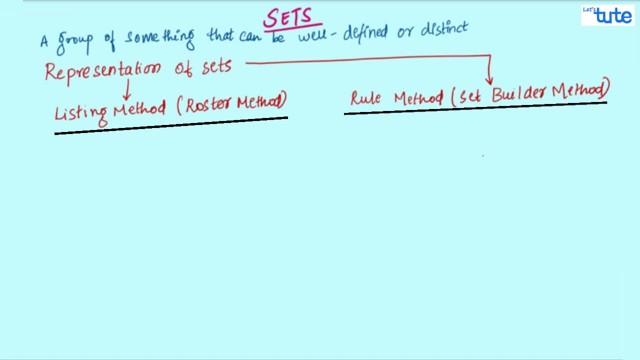 Let's see what's listing or roster method is. Let's see If I want a set of all letters in the word mathematics, then how will I write it? Well, this is a very simple method. Let's look at this in a little more detail. 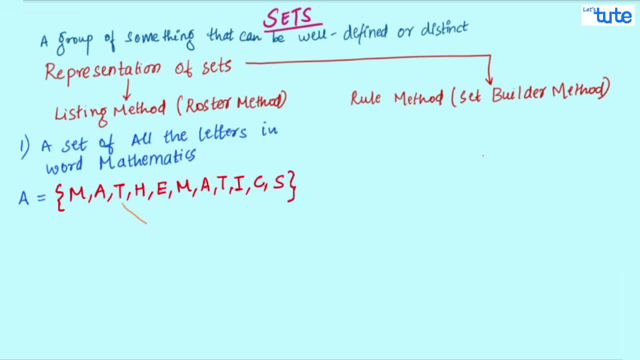 All the letters in the brace or curly brackets are known as elements A, or any letter can be used to represent this set. However, there's one tiny mistake that is there in this set. The elements in this set are never repeated. Every element appears just once in a set. 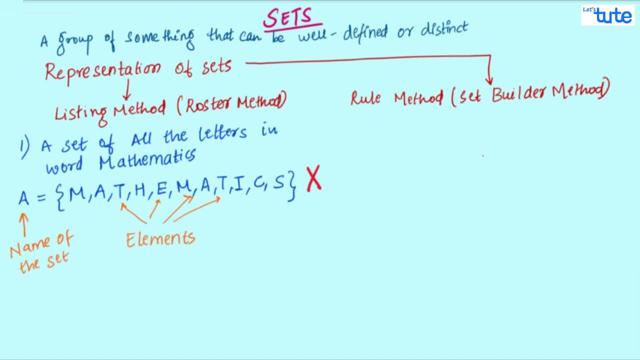 Hence, the solution of this set of all the letters in the word mathematics will be: A is equal to curly brackets. M, A, T, H, E, I, C, S, Curly brackets, closed. This is how to write a set of all the letters in the word mathematics. 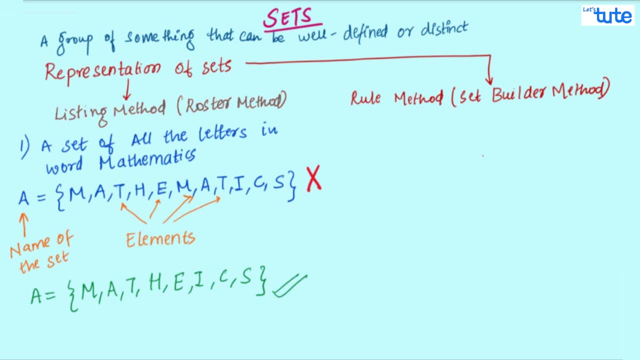 Let's see how to write a set of all the letters in the word mathematics. A is equal to curly brackets- M, A, T, H, E, I, C, S. Curly brackets- closed. Let's see This is how we present a set in a roster method or a listing method. 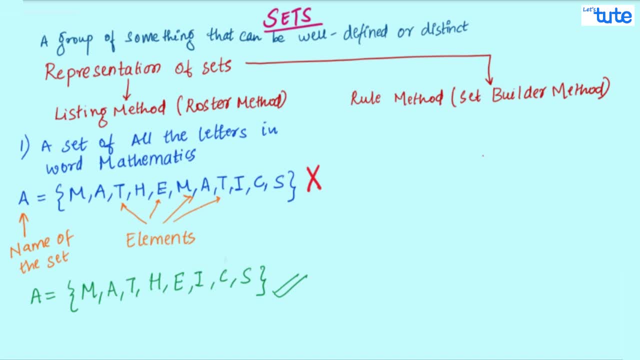 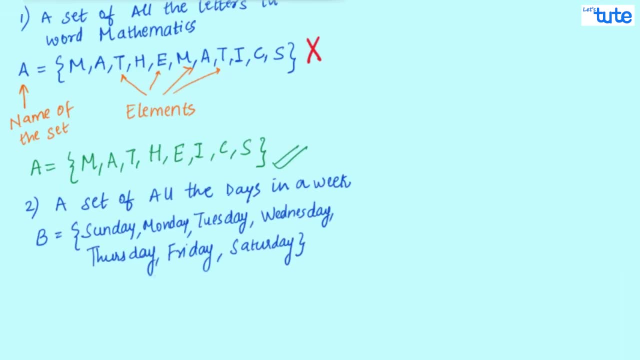 Now, since just we have listed all the letters is the reason why it is known as a listing method. Next can be a set of all the days in a week, a set of all the rainbow colors, etc. We have also been studying sets in few of our previous grades. 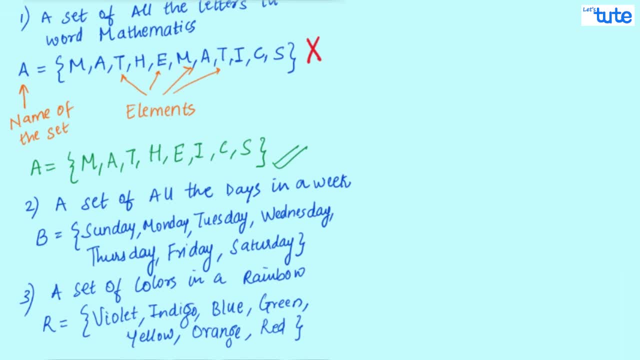 It's just that we never knew that they are sets like a set of natural numbers, A set of whole numbers, a set of integers, etc. Sets are used in a variety of places in mathematics, but we'll see that in the future sessions. 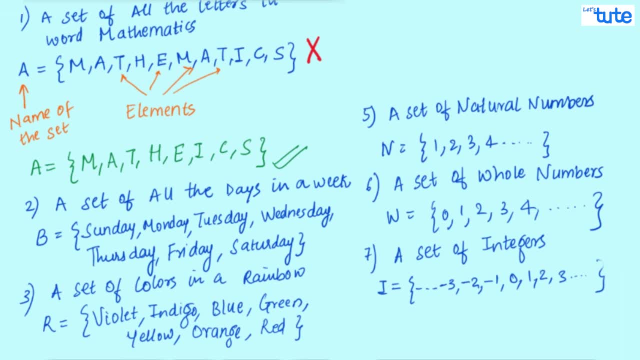 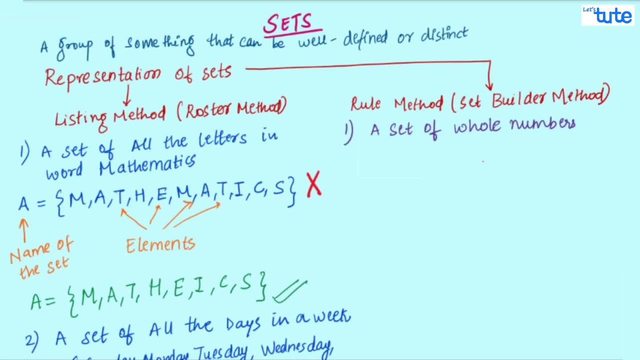 So now I believe you can make any set using the listing method. Now what happens if I ask you to form a set of all the whole numbers between 0 to 10,000.. Can we use this listing or roster method to list all these whole numbers till 10,000??